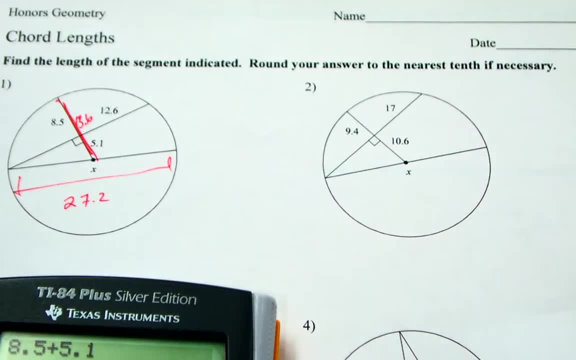 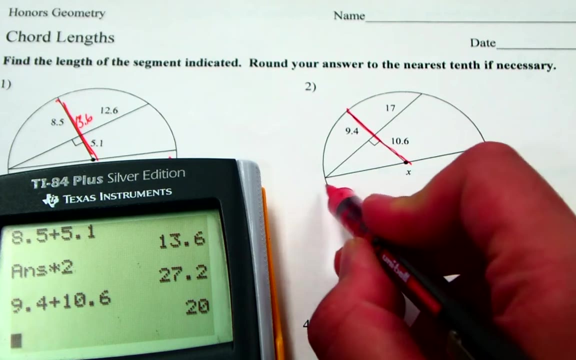 That is harder than it sounds, though. Let's take a look at the next one, Once again looking for a diameter. Hopefully, you can see that all you've got to do is find this radius length, So that would be 9.4 plus 10.6.. That's the red length, so the total diameter here would be 40.. 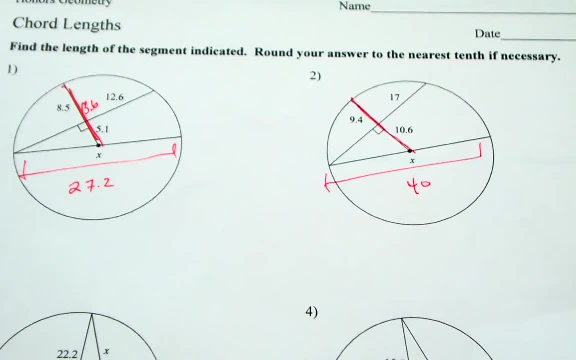 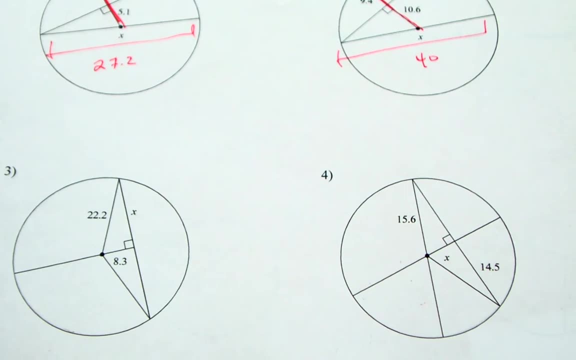 Moving along. they started off kind of easy. They're going to become a bit more complicated. So here we're given several chords, A chord, or sorry, a chord, and then a couple of radii, it looks like. So the question is, what is this length? right here It's not very clearly marked, but that's the length we're looking for. 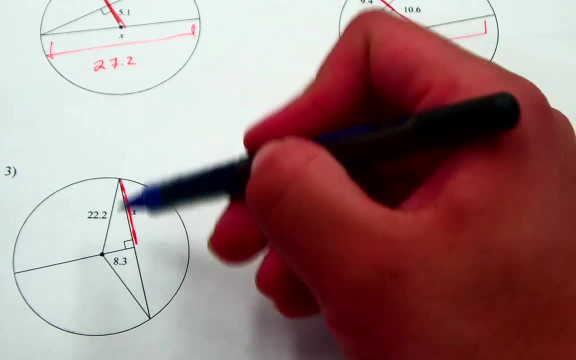 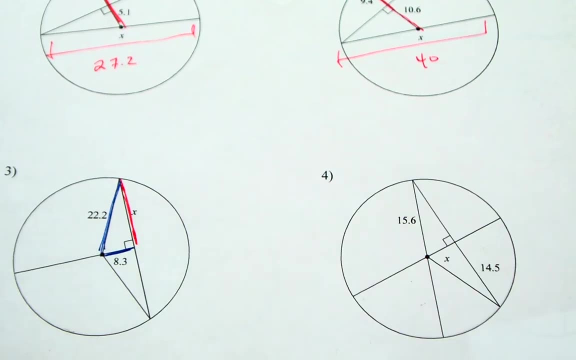 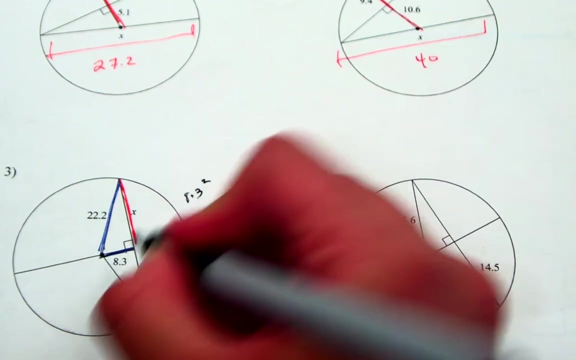 Well, hopefully you realize that this is a radius right here and conveniently it actually makes a nice little right triangle already. So all we've got to do is use the Pythagorean theorem. So that would be, let's see, 8.3 is one of our legs squared plus x squared. 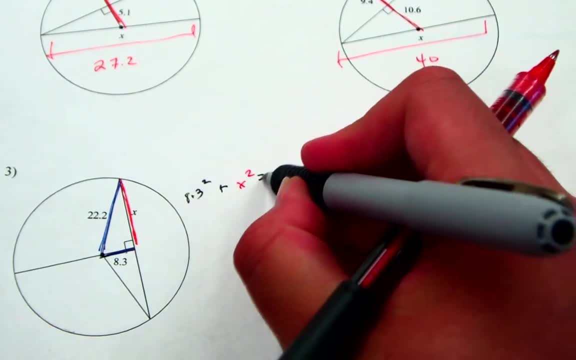 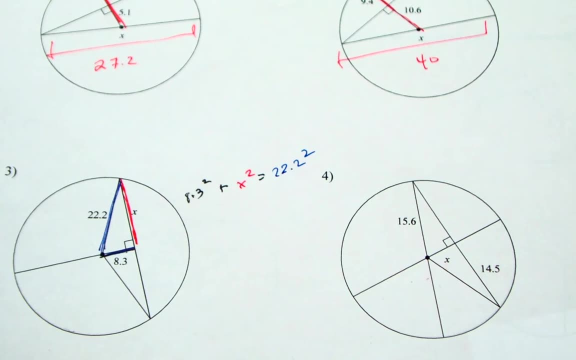 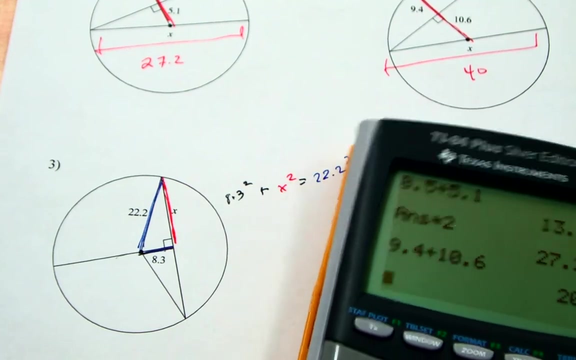 Which is the unknown length, is going to equal the blue length, the hypotenuse, which is 22.2 squared. So with a little bit of calculation we can find the value of x. So bear with me a moment, I'm just going to zoom out a bit. 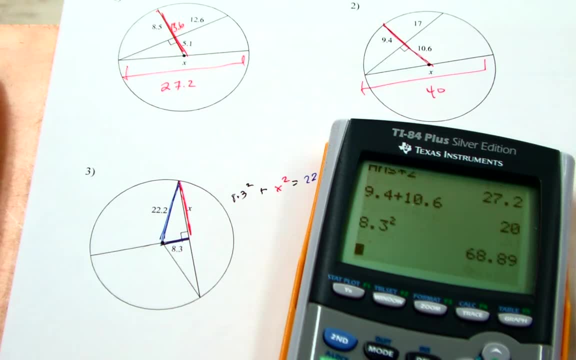 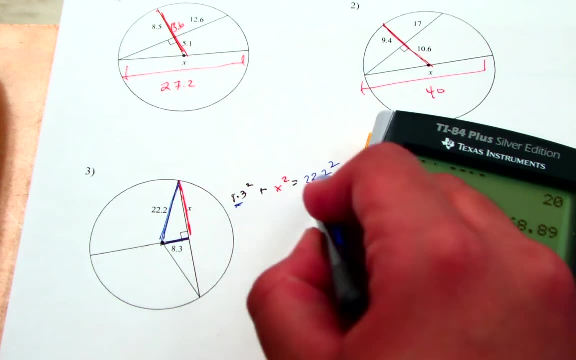 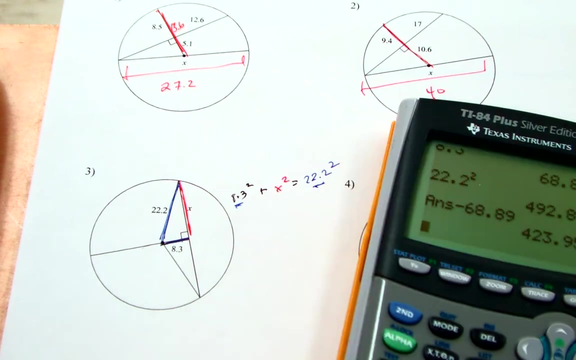 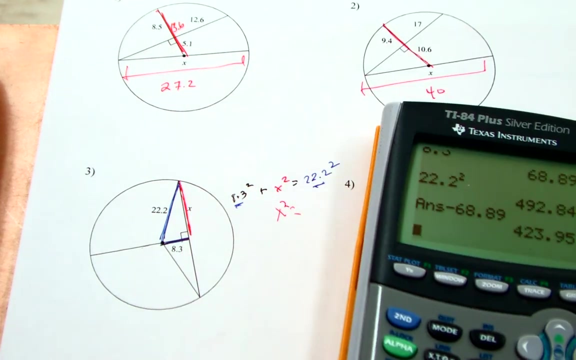 We have 8.3 squared, which is that number, 22.2 squared, which is that number I'm going to subtract. I'm going to subtract this from this. so minus this quantity, So that means that x squared is 423.95,, which means we're one step away from finding just x. 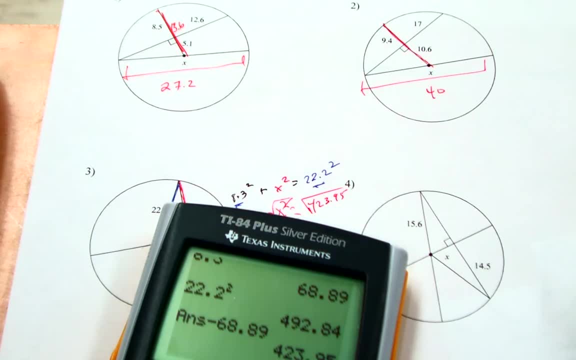 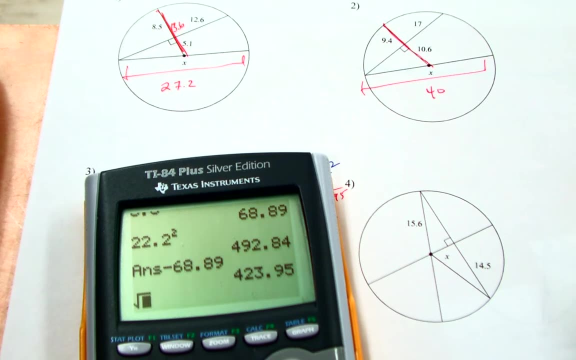 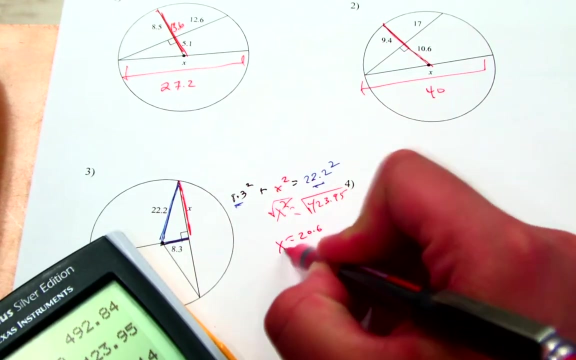 Take the square root, and thus x. is this value right here? Oops, Square root, The answer will give me 20.6, approximately. And there we have it. So part of the challenge here is recognizing when to use which particular skill. 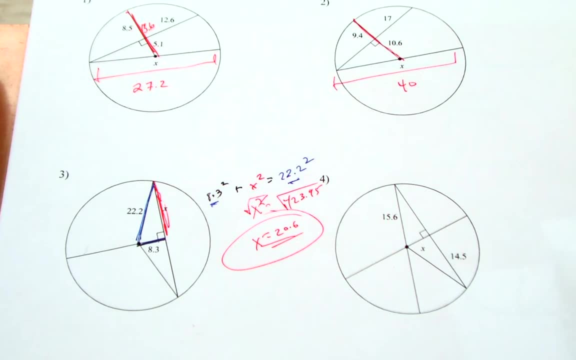 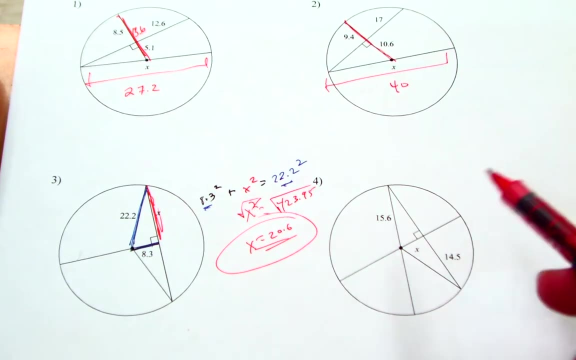 And that takes a little bit of trial and error, but some practice here, hopefully, will help you become more proficient at that. Here we're given a very similar shape in some regards. We were asked to find this length right here. It's not very clear. 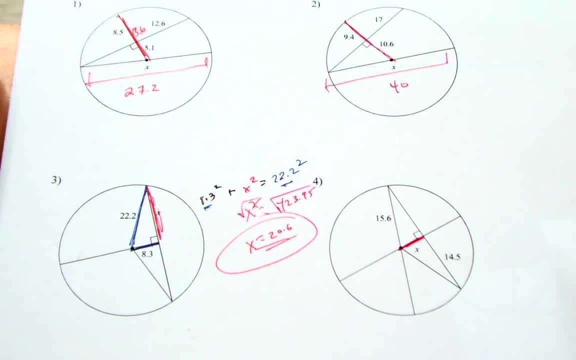 It's not very clear because of the software. Nevertheless, all we've got to do is to recognize that that length is going to be found using the Pythagorean theorem, because of this blue length right here is a radius 15.6.. 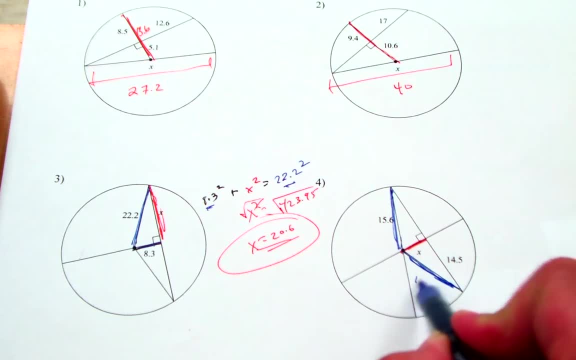 All radii in a given circle are congruent, so this is also going to be 15.6, and once again we have a very similar problem to the one before, So I'm not actually going to work this one out, but hopefully you can realize that you can carry this distance here, because they're both radii. 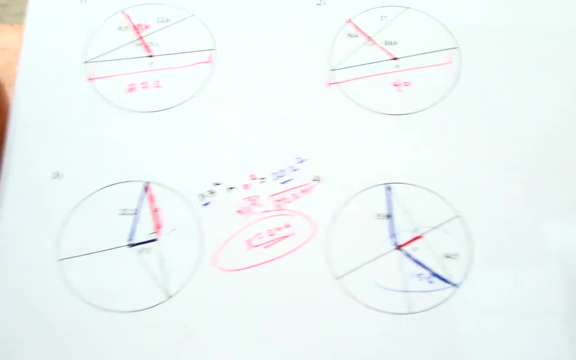 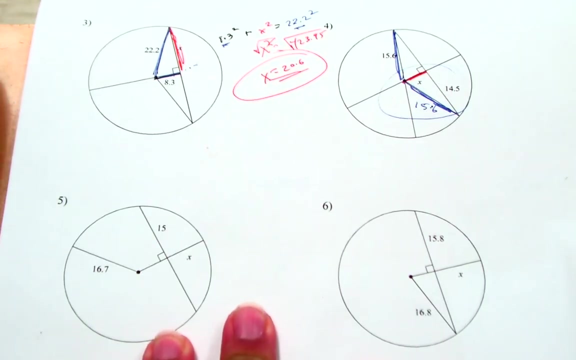 And then it's very much like this problem right over here For the last two in our set. here we're asked to find parts of radii. That requires a little more nuance. once again, Let's take a look at this first one. 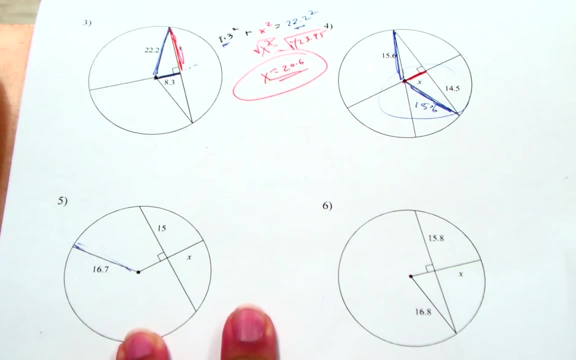 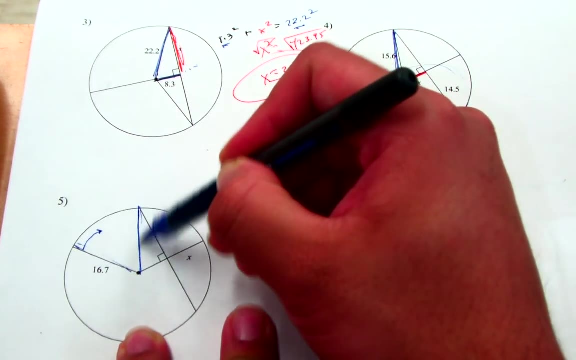 This radius length of 16.7 is not very useful where it is, so I'm actually going to basically rotate it along the circle until it becomes this length here. So these are both radii center to edges, so this would also be 16.7.. 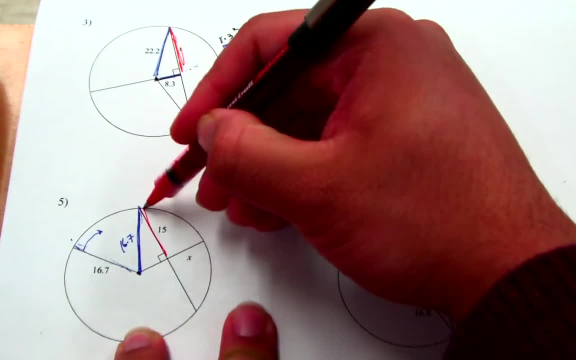 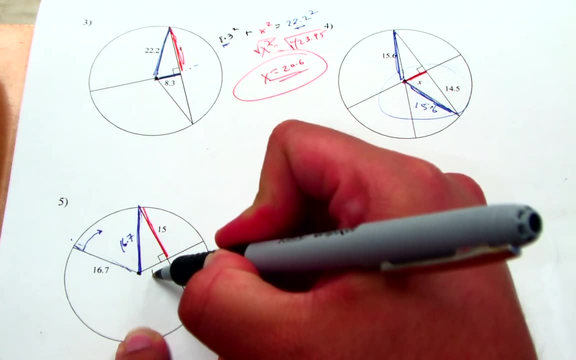 I'm given this 15,, which represents this length right here, And what I'm looking for is not really part of that. but if you think about it for a second, if I can find, for lack of a better word, let's call this b. 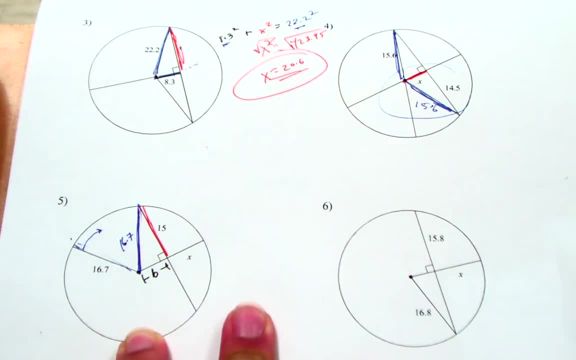 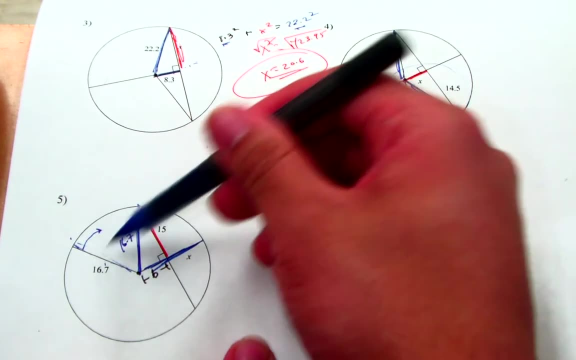 If I can find b right here, do you see how that will help me find x? Because I know that in total this length right here is also 16.7, because all three of these are radii. So if I can find b, I simply take that away from 16.7, and I will have x. 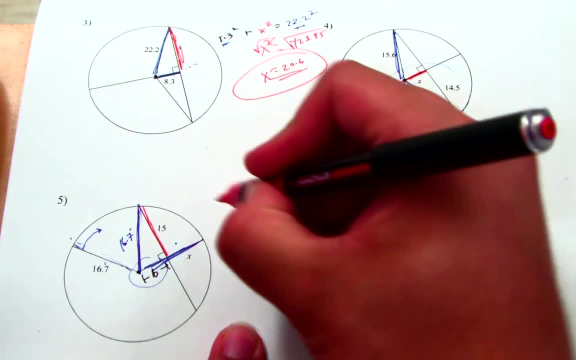 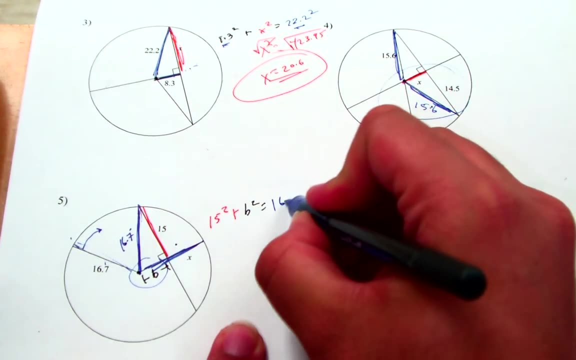 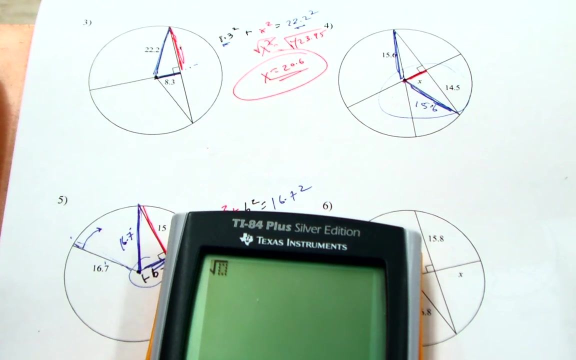 So, once again, using the Pythagorean theorem, This would be 15 squared plus b squared equals 16.7 squared. So let me show you a little shortcut in the calculator. What you can do is recognize it's going to be the square root of 16.7 squared minus 15 squared. 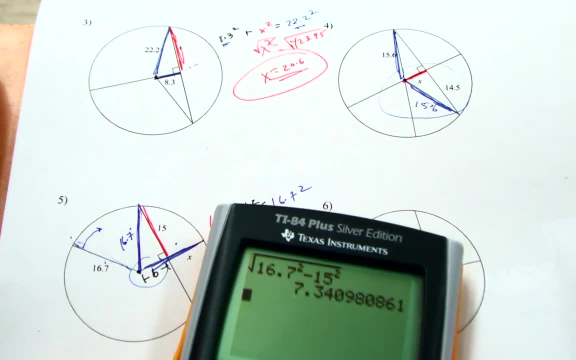 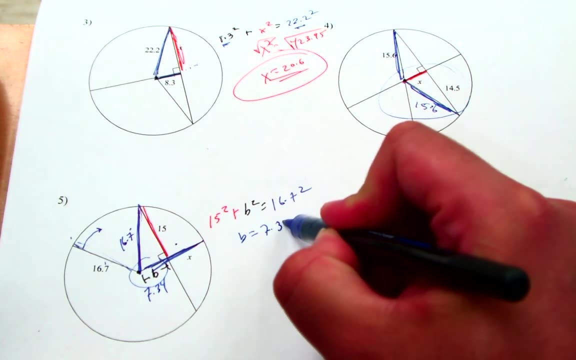 And right away we'll get 7.34.. So this length right here is 7.34.. So that's not x, but it's pretty much giving us x because we know that this whole length here, as mentioned, is 16.7.. 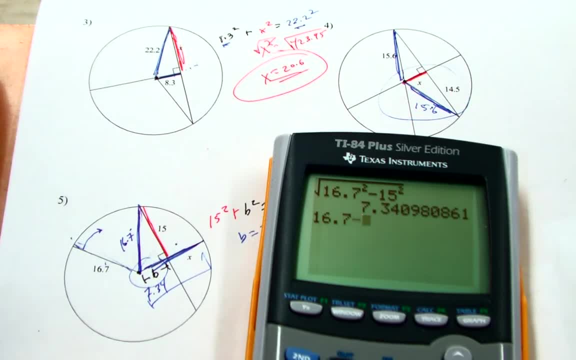 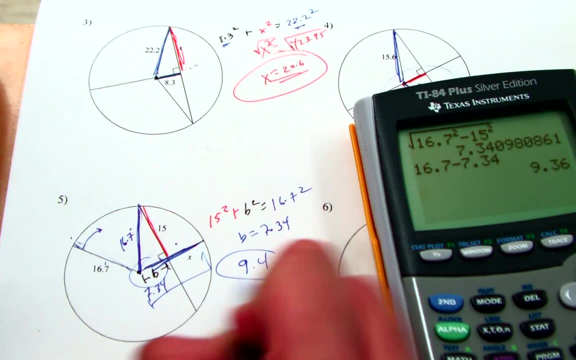 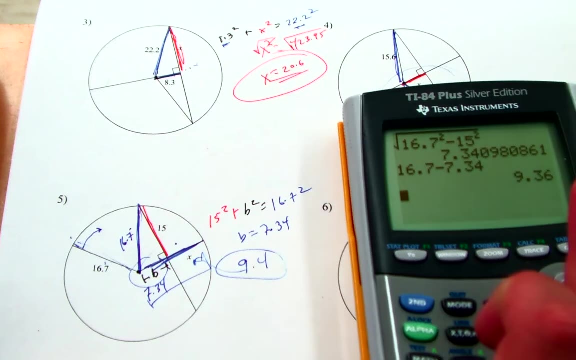 So simply take away from 16.7,, 7.34, and we have a final answer of approximately 9.44x. So a lot of moving parts there, but if you take them each step by step, you'll see it's not too bad. 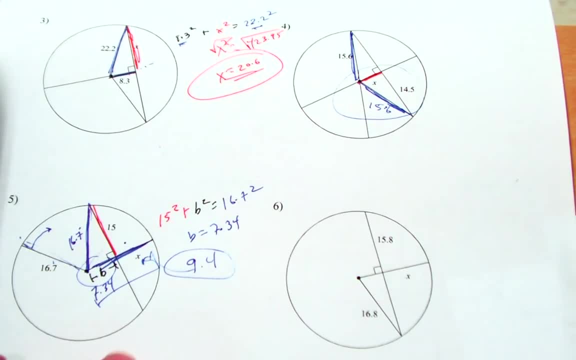 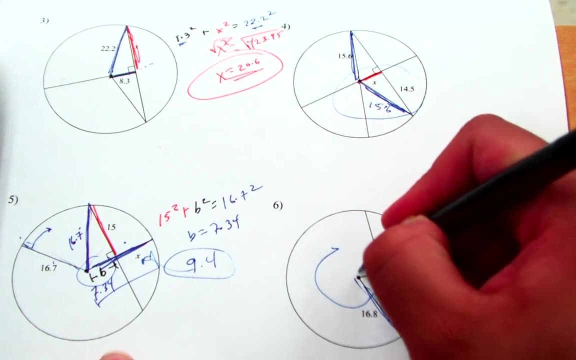 This problem here once again, is very similar. We're not going to work it out. We're not going to work it out in depth, but all you've got to do is carry the radius length around the circle so that it's here. 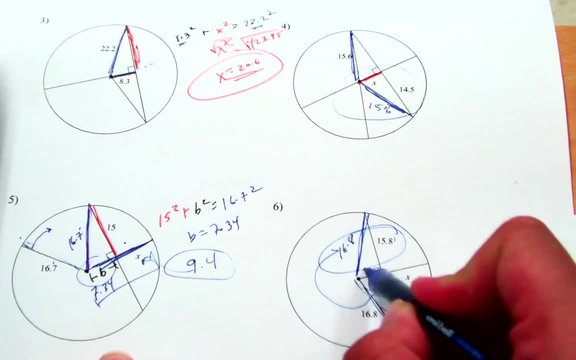 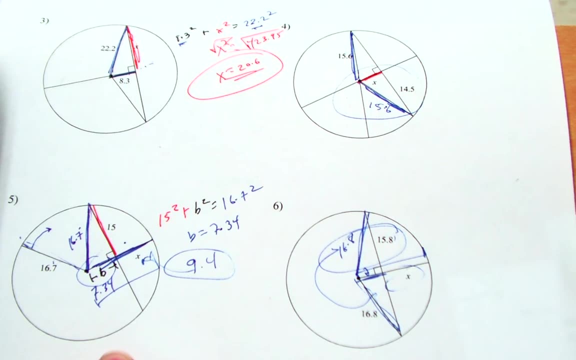 So that would also be 16.8.. Use the Pythagorean theorem of these to find this length. Remove that length from this third radius, which is also 16.8, and you will find x. So hopefully this gives you a glimpse of what to look for and what to do when you've spotted certain situations. All right, see you in class. 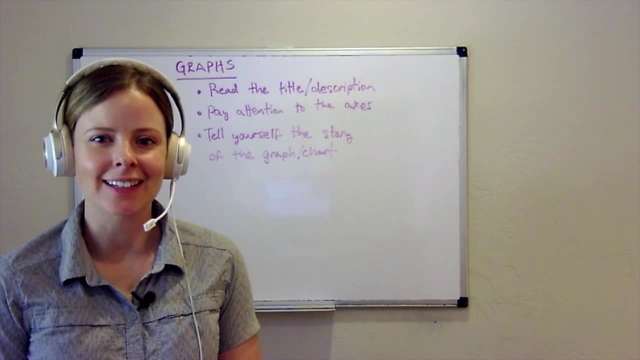 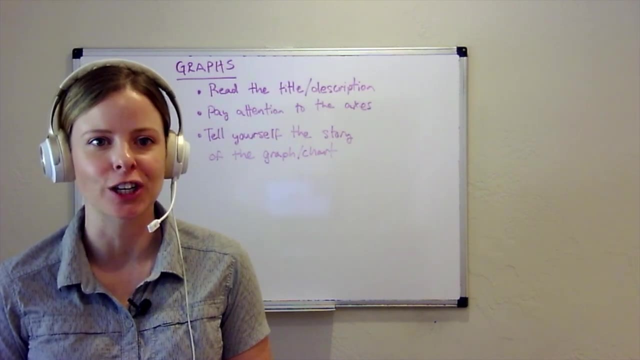 Hi, this is Dana with GMAT Ninja, and today I'm going to be talking about the graphical interpretation questions that you'll see on the Data Insights section of the GMAT. So this is just an introduction to you see these graphs, you see these charts. what do? 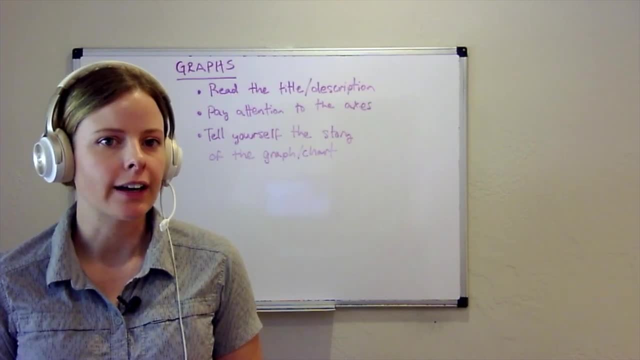 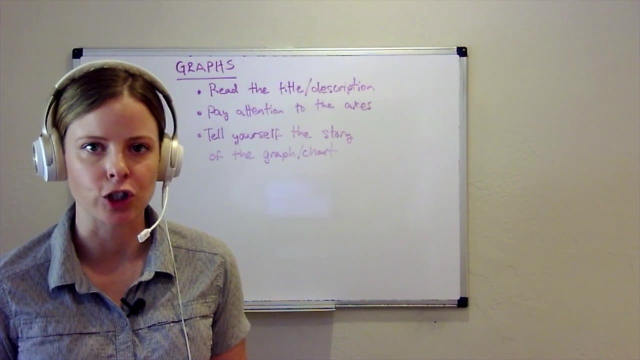 you do with them? How do you approach those kinds of questions? None of these questions that we go over in this video are going to be knock-your-socks-off difficult. We'll start with a couple of easy questions and then move into a couple of medium questions, but really 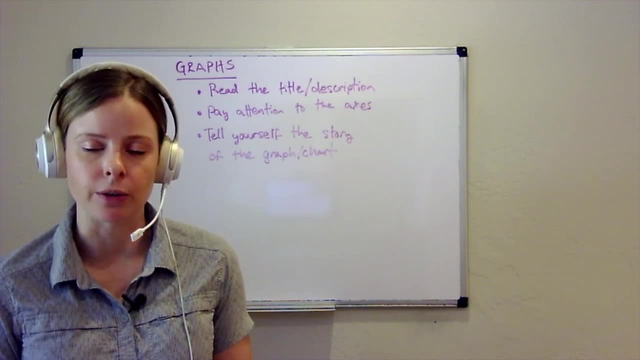 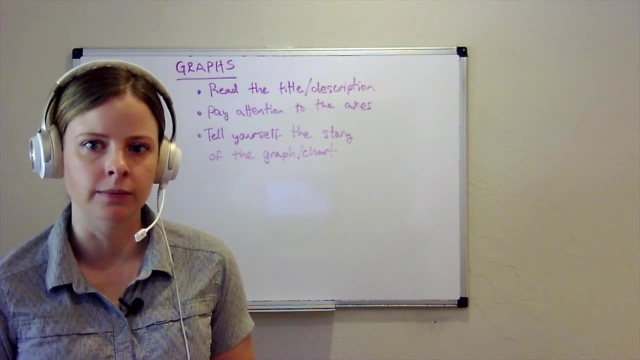 the point is just to get that overall approach down of what to do when those things pop up on the screen. We'll go over line graphs, bar charts, pie charts and flow charts in this video, which are some of the more common things that you'll see on the Data Insights. 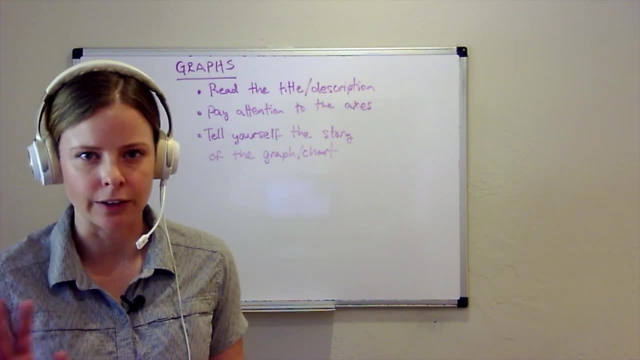 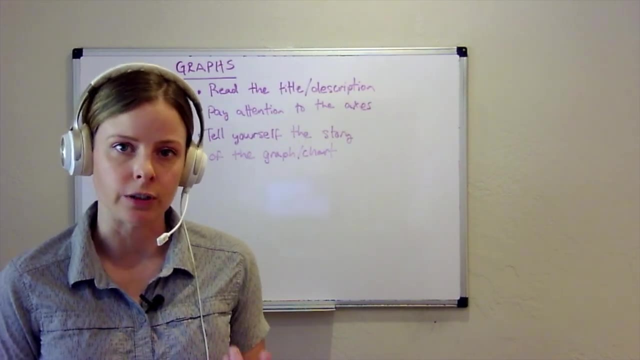 section, although you're always going to see those outlier weird graphs, and those will be covered in a different video. So, before we dive into particular questions, what is that overall approach? What should you do when you see a graph or a chart on Data Insights, The problem that we see most? 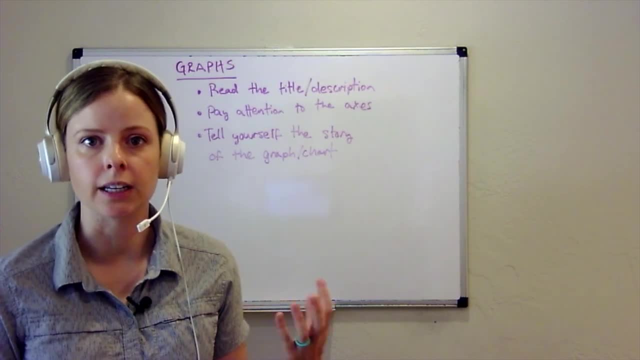 that we see most frequently with our students is that they rush into the questions before they really understand the information that is presented in the graph or on the chart. So you don't want to do that. So our approach is all about giving yourself a little bit.